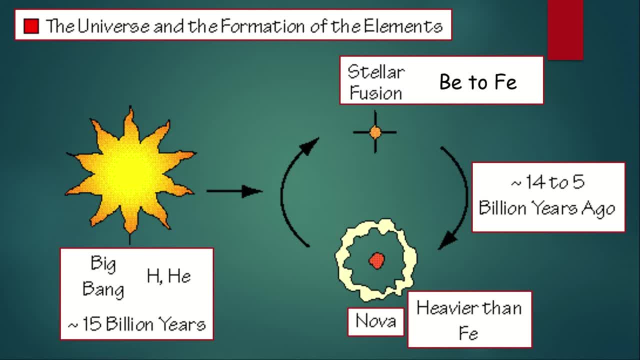 During the Big Bang. hydrogen and helium are the first elements, nitrogen finished and helium from the NaCl quantum energy form, and that happened 15 billion years ago. as the universe developed, stellar fusion occurs where in the stars are formed and during that time beryllium to 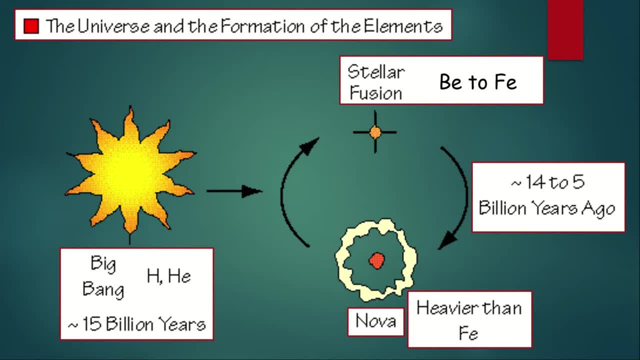 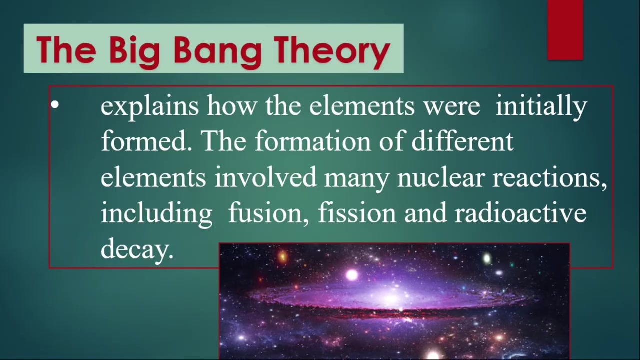 iron elements are formed. 14 to 5 billion years ago, stellar explosion or supernova happened and during supernova or stellar explosion, heavier than iron are formed, or the elements heavier than iron are formed. so this is how the elements are formed during the development of our universe. the big bang theory explains how the elements were initially formed. 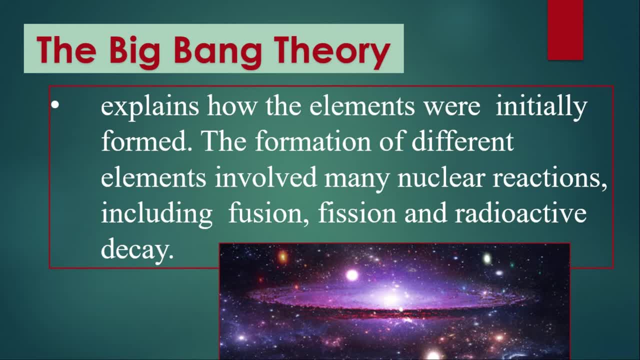 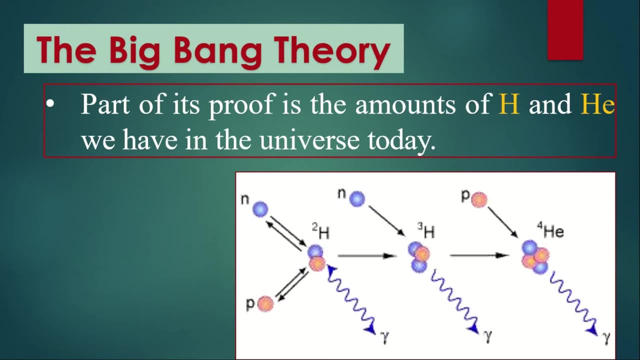 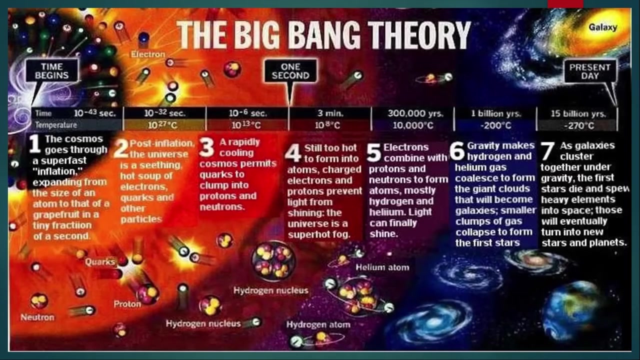 the formation of different elements involve many nuclear reactions, including fusions, fission and radioactive decay, which we will discuss on the following topics. the big bang theory. part of its proof is the amounts of hydrogen and helium we have in the universe today. this illustration shows us the evolution of the universe according to the big 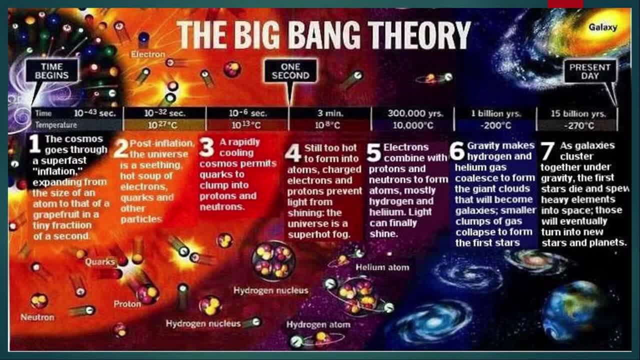 bang theory. so from time zero, from the time beginning begins until 10, raised to negative 43 seconds, all matter and energy in the universe existed as a hot, dense, tiny state, which we called the singularity. so the cosmos goes through a super fast inflation, expanding from the size of an atom to that of a grapefruit in a tiny fraction of a second. 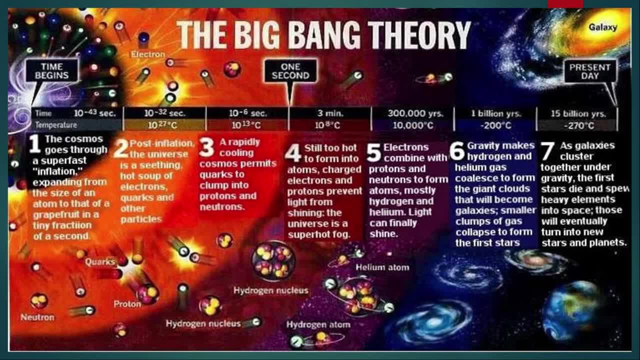 so it all started glass from a single hot, dense point, which we called the singularity. it then underwent extremely rapid inflation so it expanded our universe. from singularity it expanded from the size of an atom to that of a grapefruit. 10, raised to negative 32 seconds later. conditions allowed the existence. 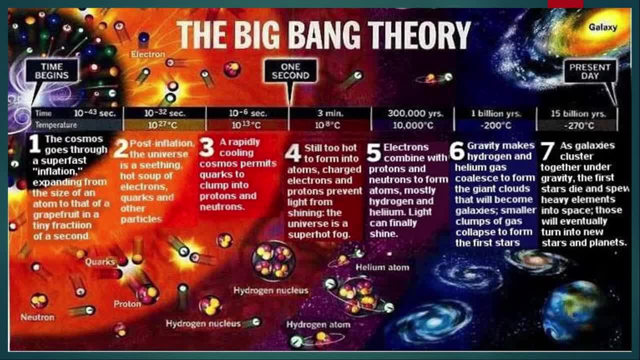 of quarks and other particles. so during that time post inflation the universe is a seating hot soup of electrons, quarks and other particles. so quarks class is a type of an elementary particle which is the major constituent of matter. is what this statement is about. in the particles we have- particles of Manhattan at 10 raised to negative 6 second- are rapidly 내용 ng. 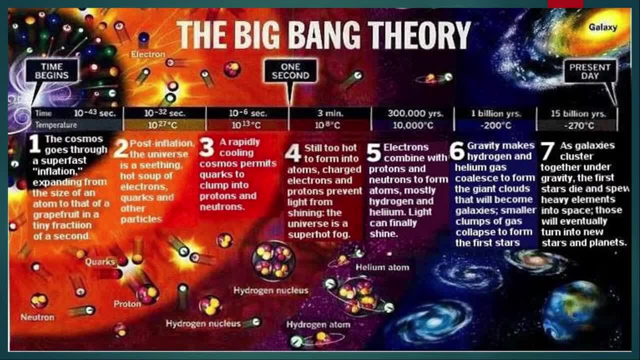 six second, a rapidly cooling cosmo-perrine じ타. It's quarks to clump into protons and neutrons. So in a tiny fraction of a second, on that part, dun palang, nag-start, magbuo, mag-clump together si quarks to form protons and neutrons. 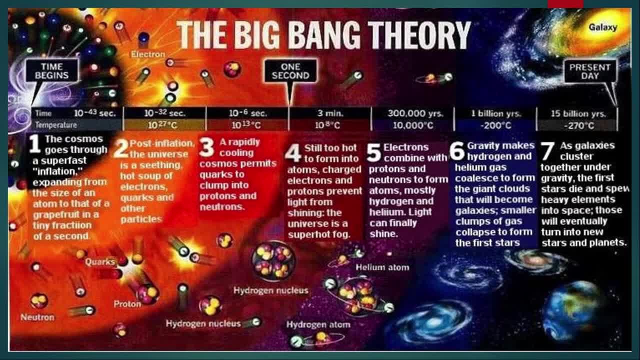 Nung lumamig ng kaunti ang ating universe And those three stages happened in the duration of one second, From the time begins to one second. yun yung mga kaganapang naganap sa ating universe. 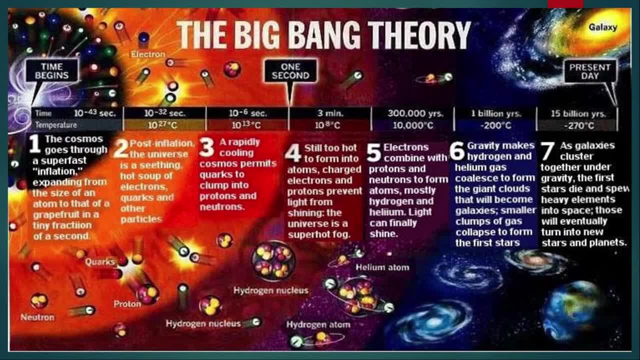 Time skipped three minutes later, So still too hot to form into atoms. So charged electrons and protons prevent light from shining. So the universe is super hot fog. So during that time there was no light. So it is also called the dark ages of the universe. 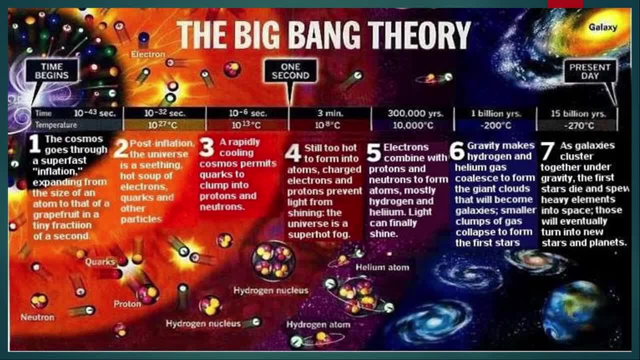 Okay, And from that point, dito na nga mag-i-start yung nucleosynthesis. So from here time skip ulit 300,000 years later, medyo lumamig na ngayon yung universe natin. 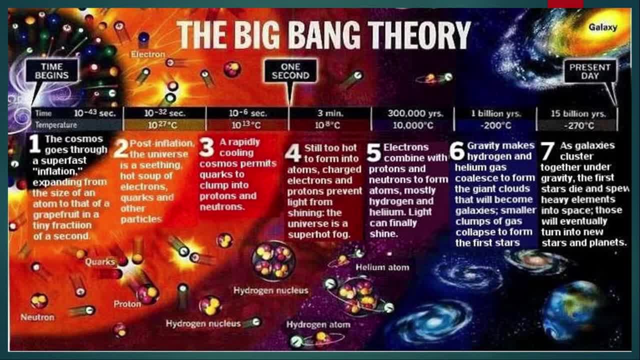 So electrons combined with protons and neutrons to form atoms, Mostly hydrogen and helium. So light can finally shine. So after 300,000 years later, palang nag-nabuo sila, hydrogen and helium. Billions of years later, gravity makes hydrogen and helium gas gawal-esk. 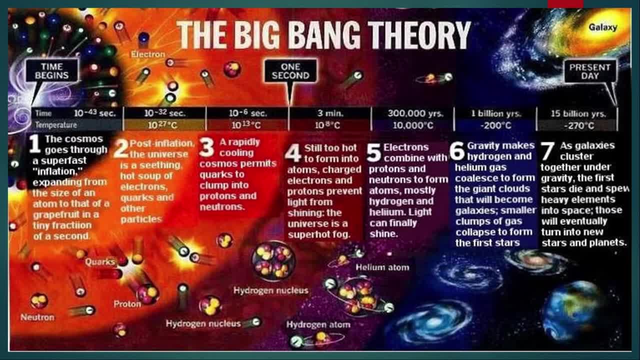 It means to clump together to form the giant clouds that will become galaxies. Smaller clumps of gas collapse to form the first star. So billions of years later pa nag-start mabuo, yung mga galaxies and yung mga stars natin sa ating universe. 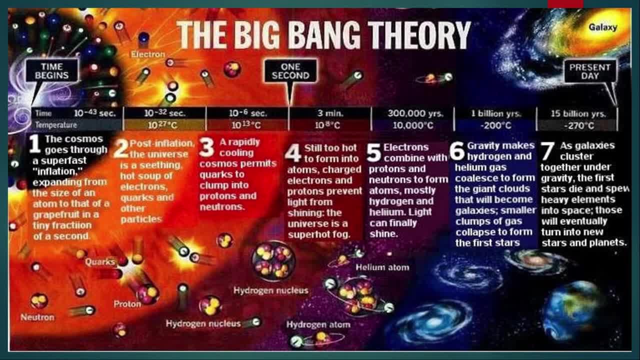 And then 15 billion years later up to the present, As galaxies cluster together under gravity, the first stars die and spill heavy elements. So dito nag-anap yung part ng stellar explosion. Pag namatay yung stars, nakakaroon ng stellar explosion or supernova, wherein nafoform yung heavy elements. 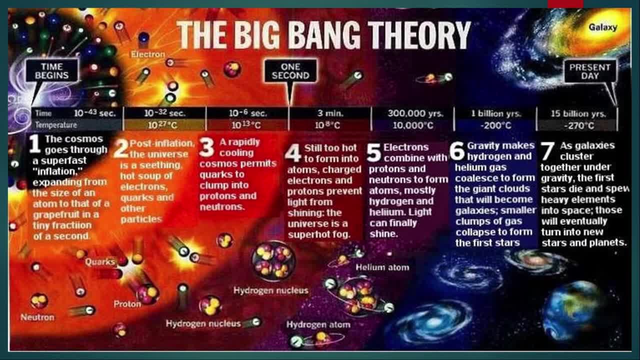 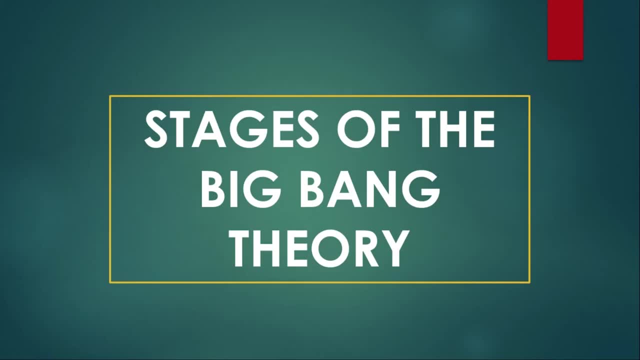 Which is na-brought out sa space. So that's how the universe evolved, From the time begins Up to the present day, According to the Big Bang Theory. So let's move on to the stages of the Big Bang Theory. So, a while ago, we have seen how the universe evolved. 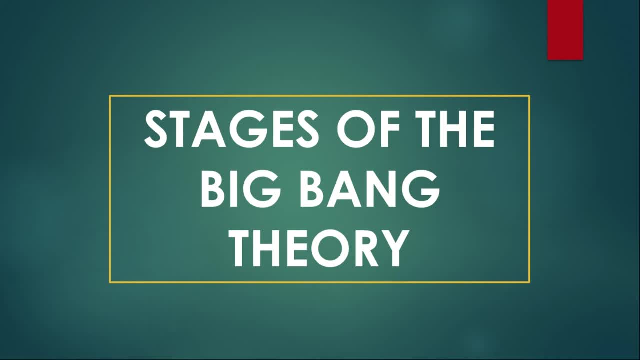 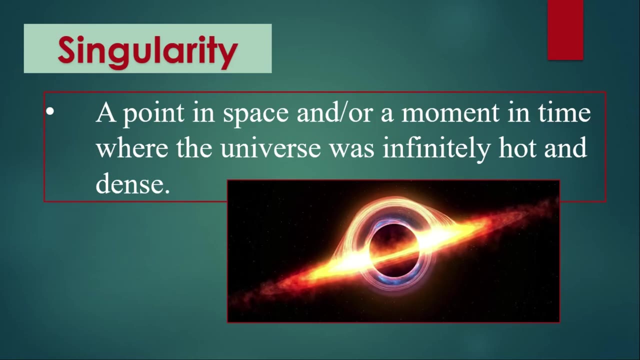 Now the development of our universe From the time, from the beginning, up to the present. Now let's go deeper on the stages of the Big Bang Theory. First we have the Big Bang Theory. First is the singularity. So, like what I have said a while ago, 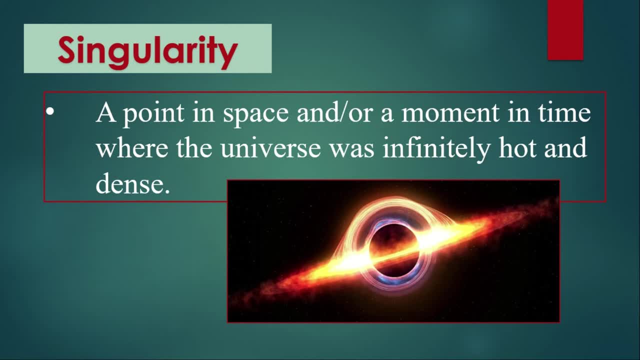 Singularity is a hot, tense, tiny state Which is also in the size of an atom. Now, this singularity is a point in space And or a moment in time Where the universe was infinitely hot and tense. So doon nagsimula ang lahat. 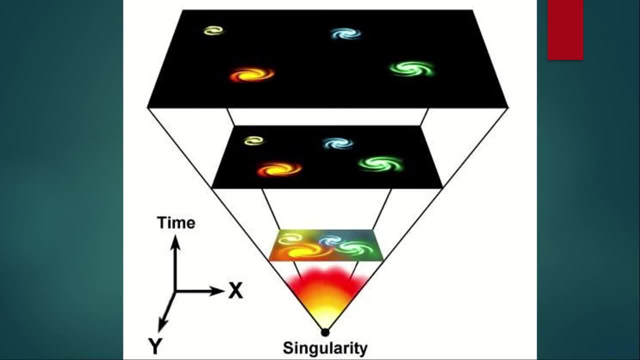 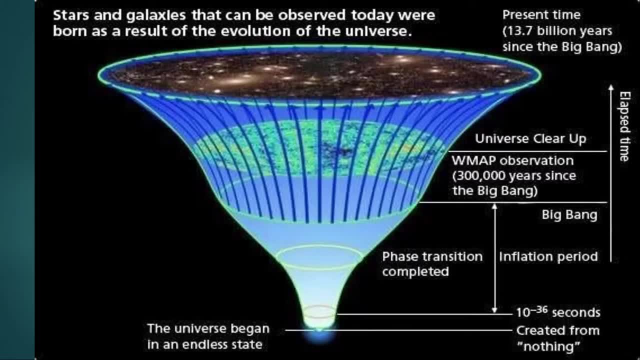 From a singularity, And then that singularity expand, An extremely rapid expansion, Which we call inflation. So here is another illustration that shows us How it all started. And then, from the singularity, Inflation happened, So it rapidly expanded. 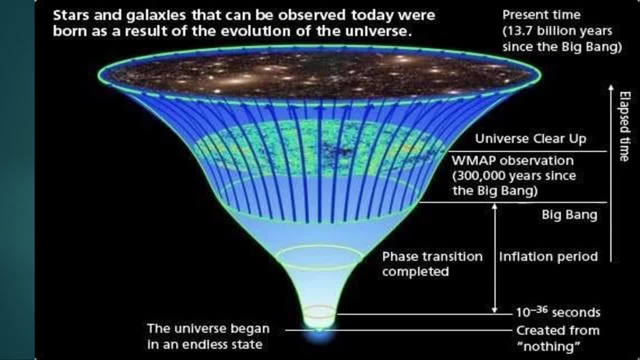 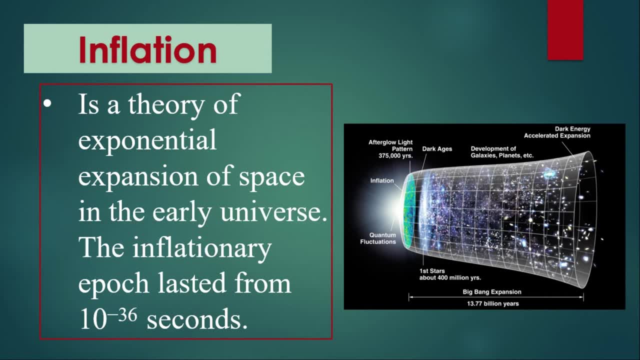 And developed into the universe That we know today. So the next one is inflation. So, as I have said, Inflation is a rapid expansion Of the universe. So it is a theory of Exponential expansion of space In the early universe. 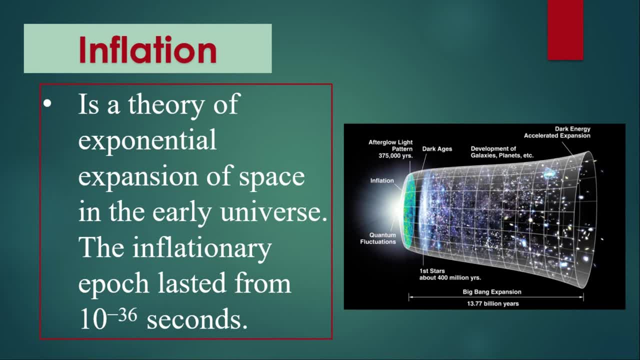 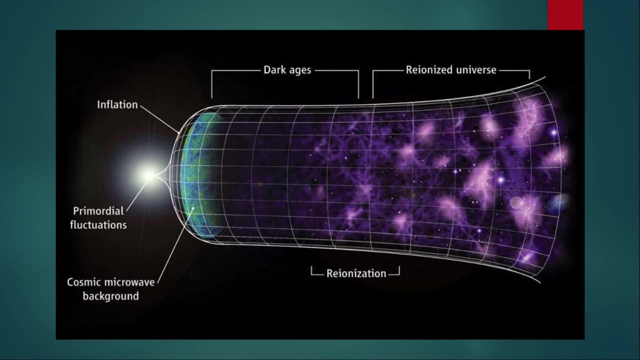 The inflationary epoch Lasted from 10 raised to negative 36 seconds. So in a tiny fraction of a second, Inflation happened. So here again Is an illustration that shows us The Big Bang, The development or the evolution. 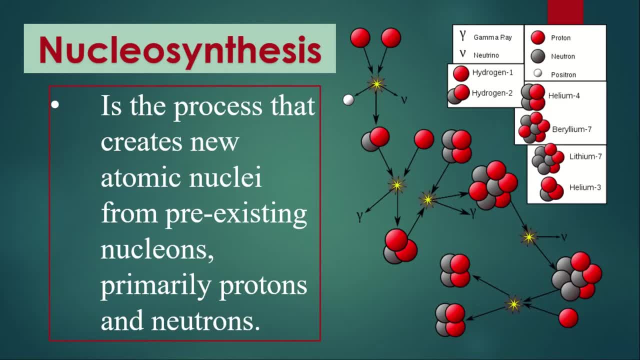 Of our universe. Now let's move on to nucleosynthesis. Nucleosynthesis Is the process That creates new atomic nuclei From pre-existing nucleons, So primarily protons And neutrons, If you can still remember class. 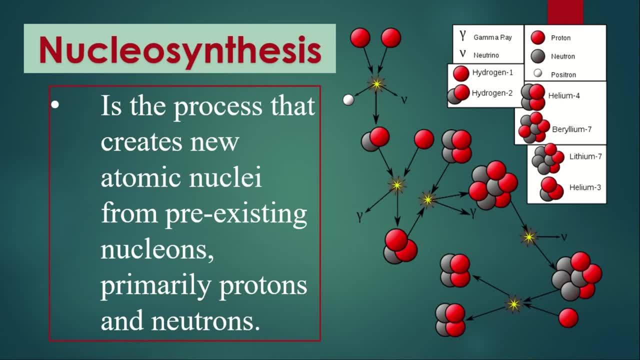 During our chemistry. subject: The nucleus Is composed of protons And neutrons. That is what forms the nucleus Of an atom. So during nucleosynthesis, In this process, The formation of Nucleos Of our atoms. 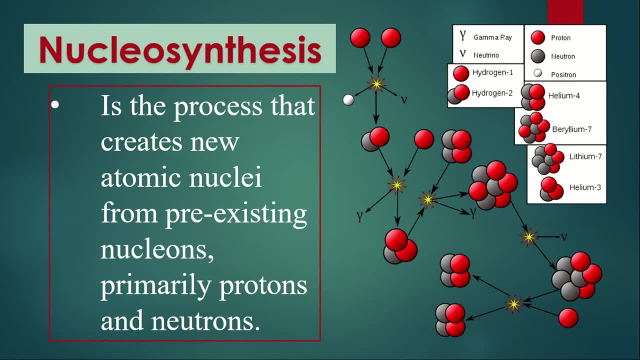 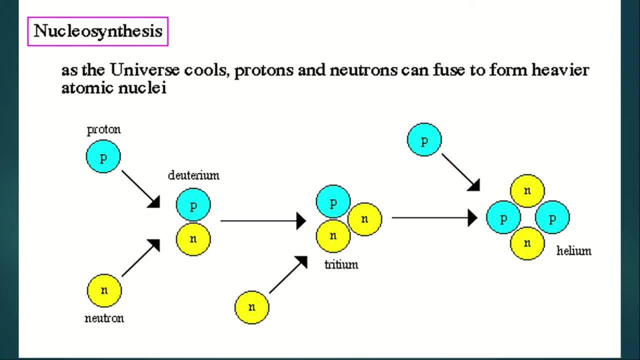 So the first Nucleos Is the nucleus of hydrogen And helium, So from protons and neutrons They combine together, Forming the nuclei. Atomic nuclei are the nucleus, So nucleosynthesis. As the universe cools, 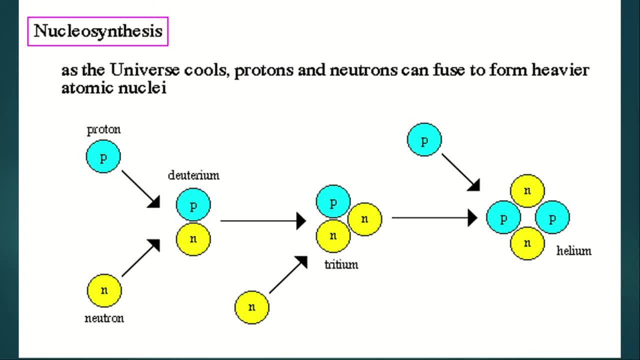 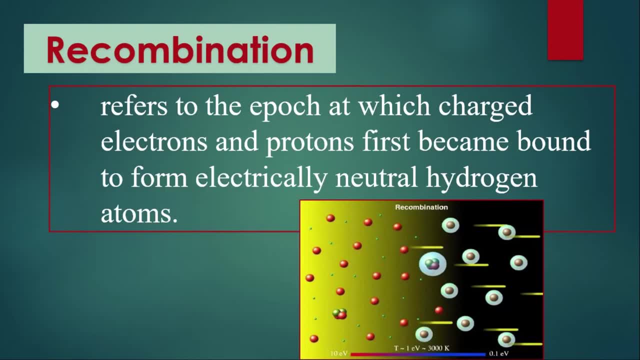 Protons and neutrons Fuse To form heavier Atomic nuclei. Recombination Refers to the epoch At which charged electrons and protons First become bound To form electrically neutral Hydrogen atoms. So during recombination. 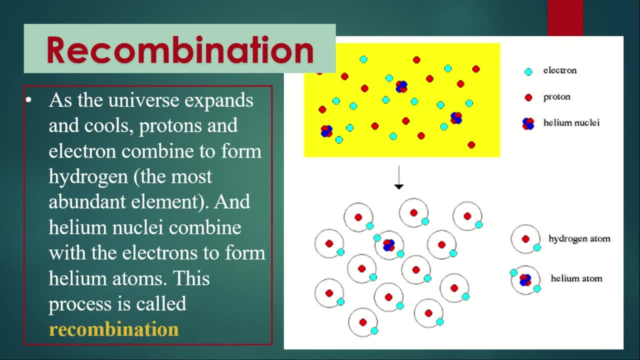 As the universe expands And cools, Protons and electrons Combine to form hydrogen, So the hydrogen atom, The most abundant element In our universe, And helium nuclei Combined with electrons To form helium atoms. So this process is called. 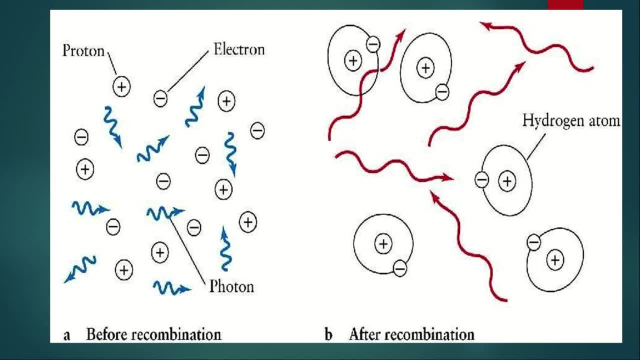 Recombination. So again here This illustration shows us Before the recombination. So we have The protons and electrons Now present in our universe That time So nucleosynthesis happened Continuously happening After recombination. 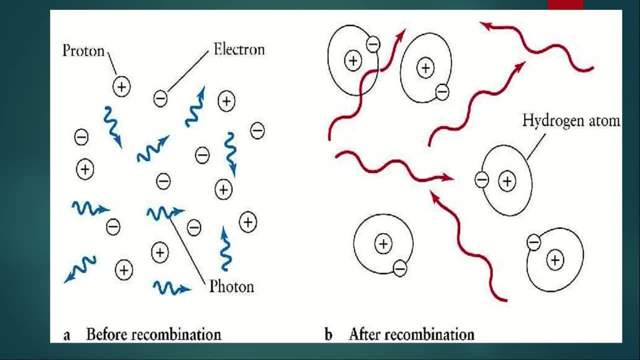 They form atomic nuclei And then they combine The protons, electrons and the nucleus Forming our atoms, Or the hydrogen and helium atoms. So after recombination There is a presence of Hydrogen atom And the helium atom. 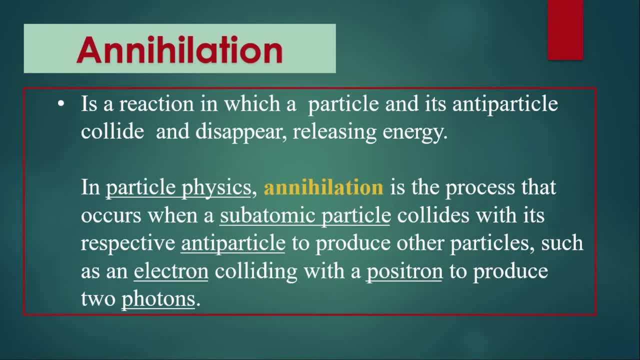 Next is Annihilation. So annihilation is a reaction In which a particle And its antiparticle Collide and disappear, Releasing energy. In particle physics, Annihilation is the process that occurs When a subatomic particle 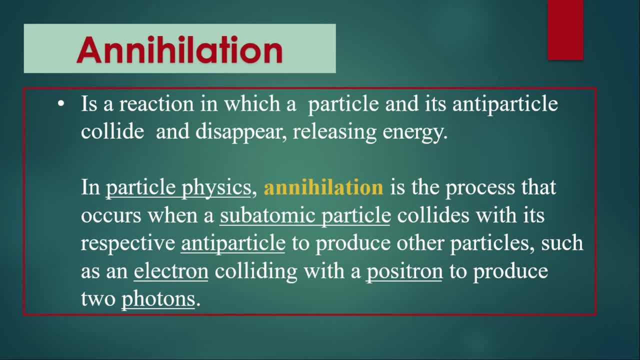 Collides with its respective Antiparticle To produce other particles, Such as an electron colliding With a positron To produce two photons. So In our universe During that time, Subatomic particles And antiparticles. 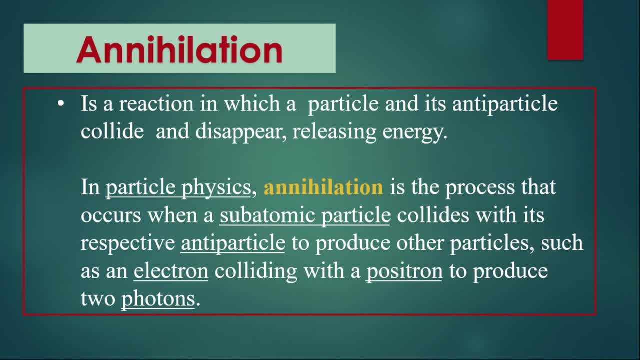 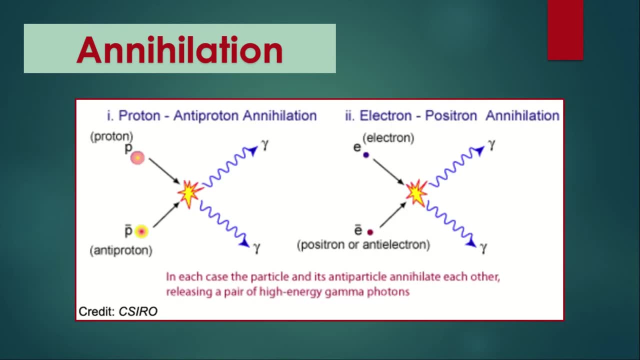 So what do they refer to? Subatomic particle And antiparticle And the process that they went through Through annihilation. Okay, So what we refer to Subparticles are the protons And electrons, So our subparticles. 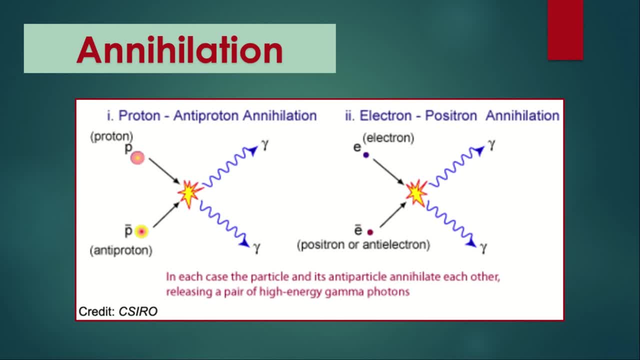 Protons and electrons. They have a counterpart, Antiparticle. Okay, So the antiparticle of a proton Is an antiproton Annihilation, And for electrons We have an antiparticle Which we call positron. 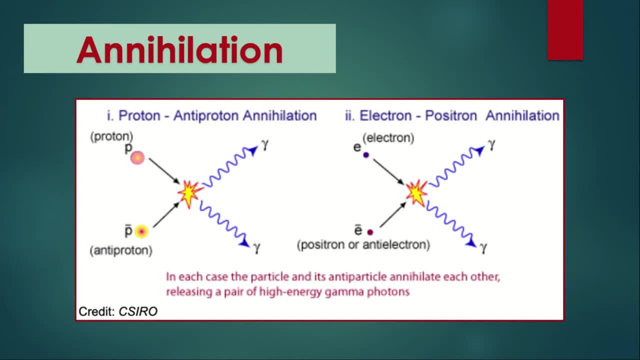 So, as we said earlier, During annihilation, This process, What happens here is that The subparticle And the antiparticle collide. So when these two collide, It releases Photons, It releases energy. So in each case, 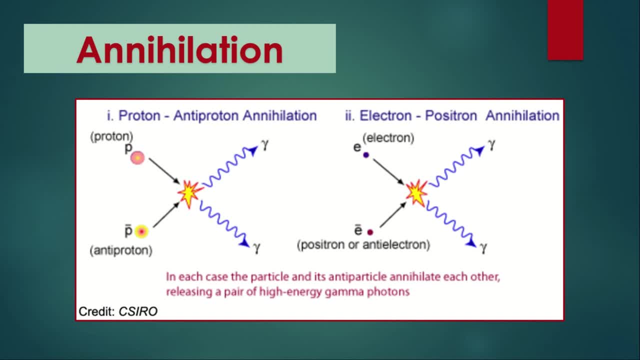 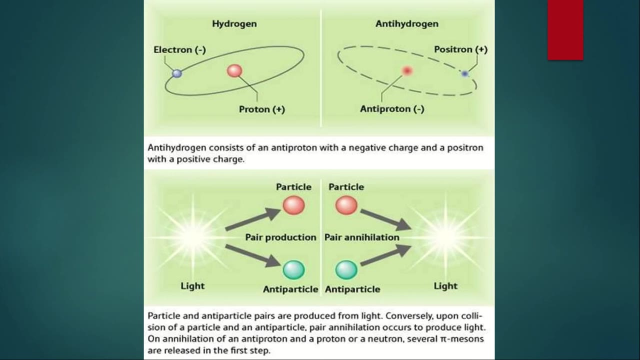 The particle and its antiparticle Annihilate each other. When we say annihilate Collides each other, It releases the pair of high Energy gamma photons. So it releases energy. So here is another illustration That shows us. 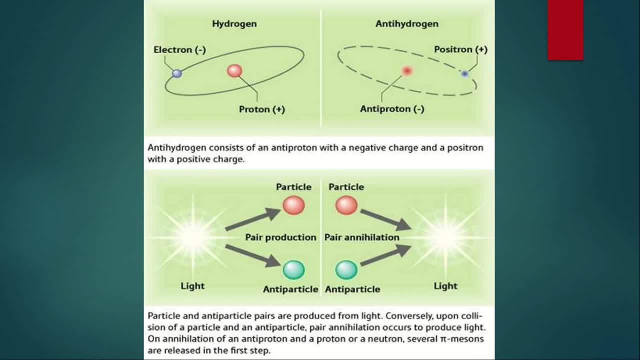 The process of annihilation, So the particle And the antiparticle pairs Are produced from light. So, conversely, Upon colliding, Or upon collision Of a particle and antiparticle, Per annihilation Occurs to produce light, 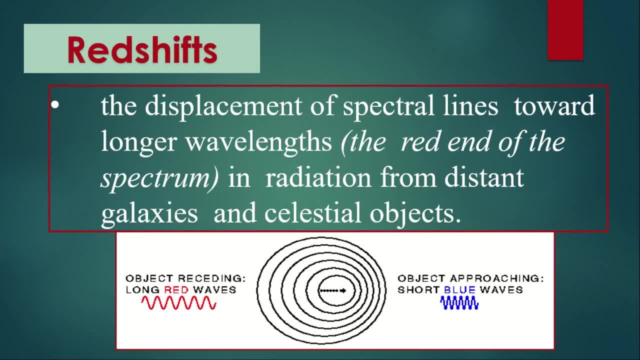 So that light, It is energy. Now let's talk about redshifts. So redshifts Is the displacement of spectral lines Toward longer wavelengths, So the red end Of the spectrum In radiation From distant galaxies And celestial objects. 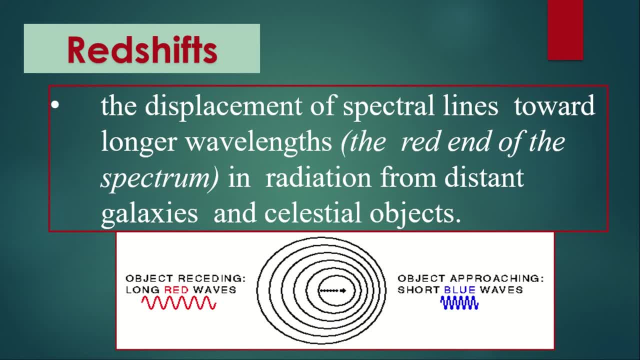 So redshift glass Is one of the evidence That proves that Big bang theory, And The red end of the spectrum here Is the red wavelength Of light That is seen And was observed by our scientists. So What does this redshift mean? 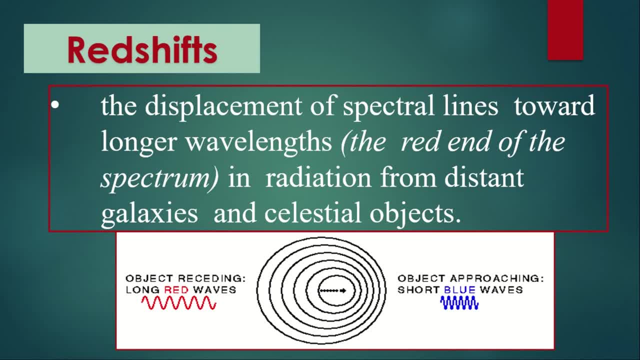 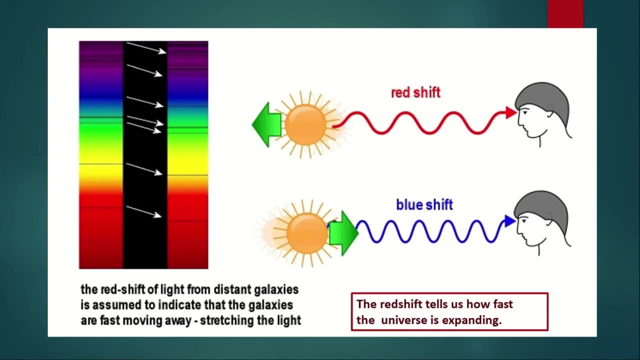 So When an object is receding. So when an object is receding, Long red waves Are observed. If an object Is approaching, Short blue waves Are observed. So the redshift of light From distant galaxies Is assumed to indicate. 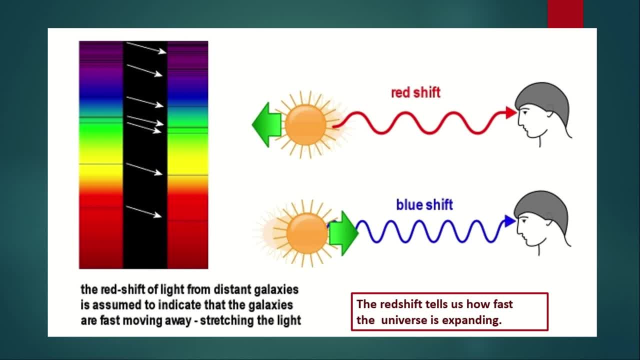 That galaxies are fast moving away. So the light stretches By stretching the light. So the redshift tells us How fast the universe Is expanding. So this is observed by our scientists For the past years, The wavelength of light That they observed from our universe. 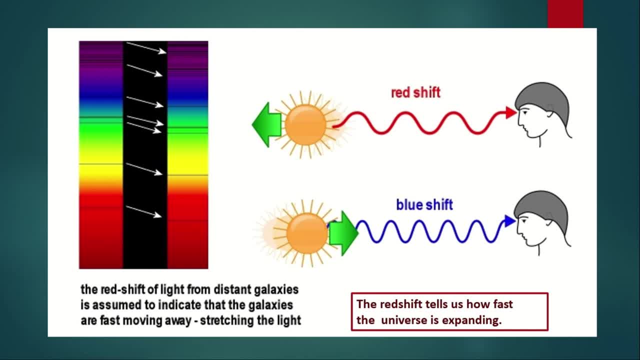 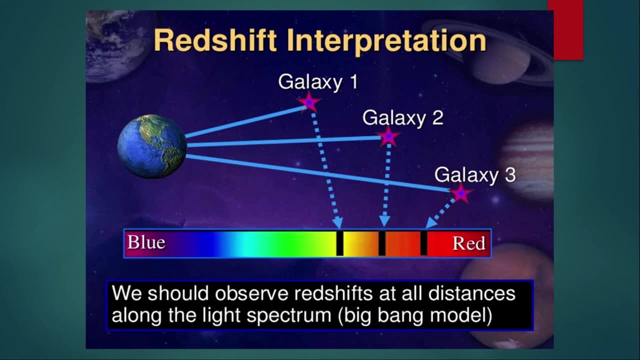 From the galaxies Around us. They noticed that this is shifted Towards the red wavelength Of the spectrum, And it means that the galaxies Are moving away from us. So that's why The redshift Becomes one of the evidence. 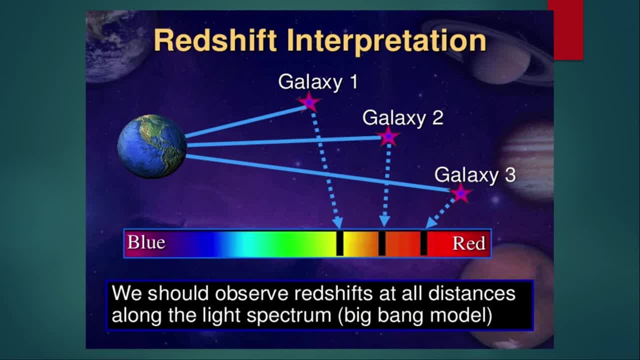 That proves That the universe Is really expanding. It was observed by the scientists. They noticed that The neighboring galaxies Are getting farther and farther Because the redshift Is shifting towards the red, The wavelength of light That is perceived. 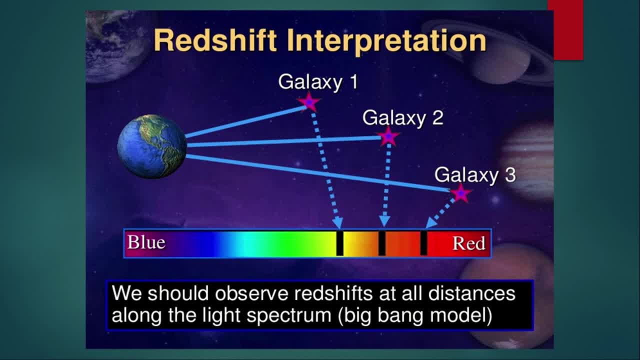 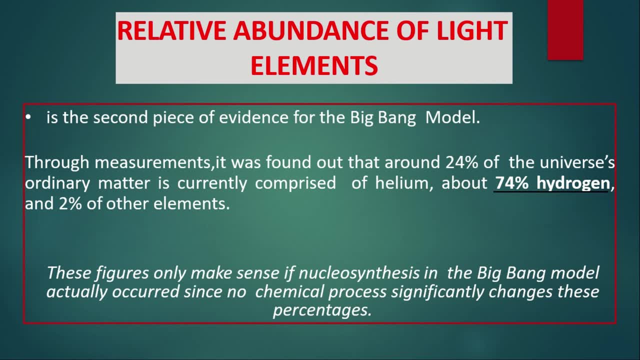 So that means That the universe Is really expanding. Another evidence That proves the big bang theory Is the relative abundance Of light elements. So this is the second piece of evidence For the big bang model. So through measurements It was found out. 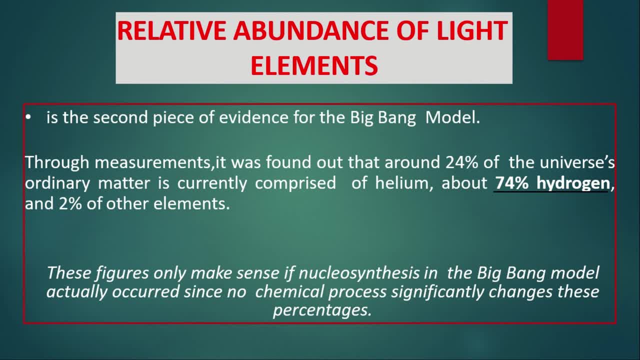 That around 24% of the universe Ordinary matter Is currently comprised of helium. So 24% helium And about 74% Hydrogen, And only 2% of Other elements. So relative abundance of light elements Is the evidence. 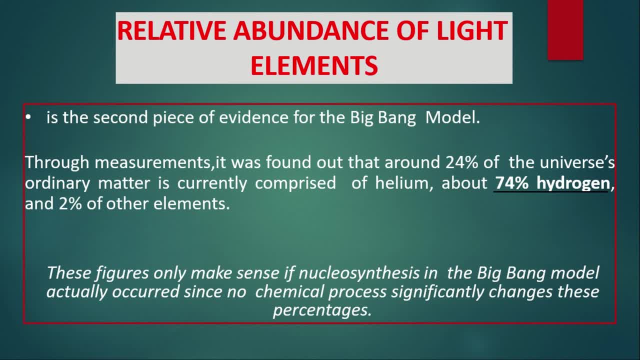 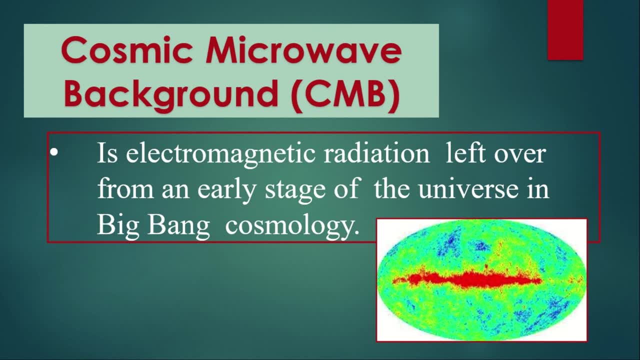 That proves, or one of the evidence That proves, the big bang model. Next is Cosmic microwave background. So cosmic microwave background Is another evidence That proves the expanding universe, That proves that the big bang Happened. It is an electromagnetic 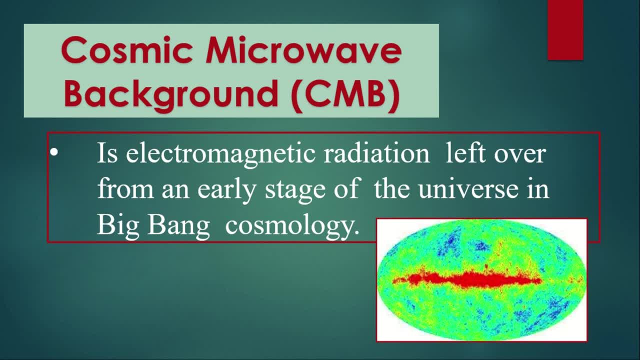 Radiation left over From an early stage of the universe In big bang cosmology. So, as I have explained a while ago, During the formation of the elements The particles of matters Fuse, Combine, Collides, So those things happen. 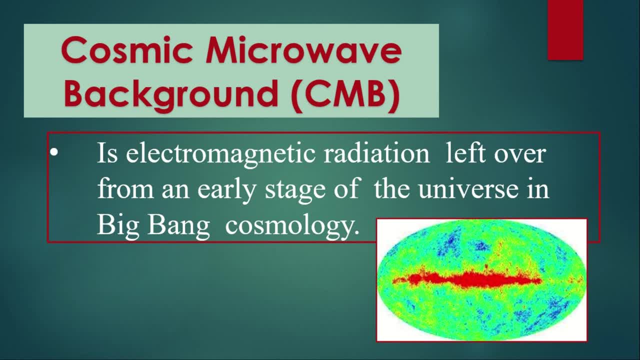 And when those particles Collides, Fuse Light is released And that energy becomes A left over or a radiation Left over. So, and that is what We known today As the cosmic microwave Background, So it is the radiation left over. 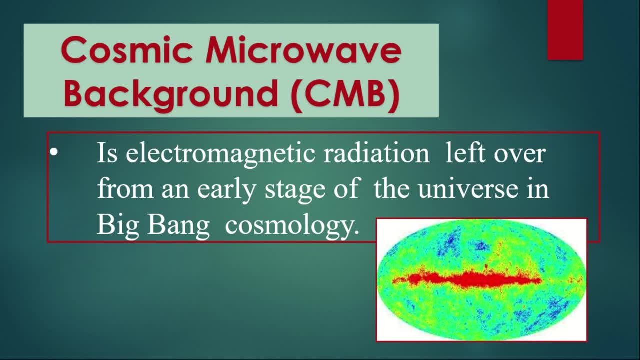 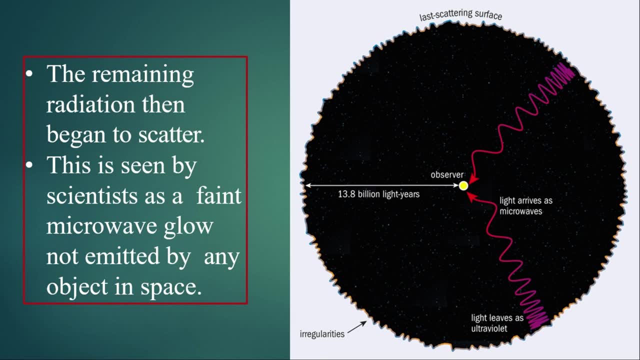 From the early stages Of the development Of our universe. So the remaining radiation Then began to scatter, And this is seen by Scientists In the microwave glow, Not emitted by any object In space. So it is just scattered in our universe. 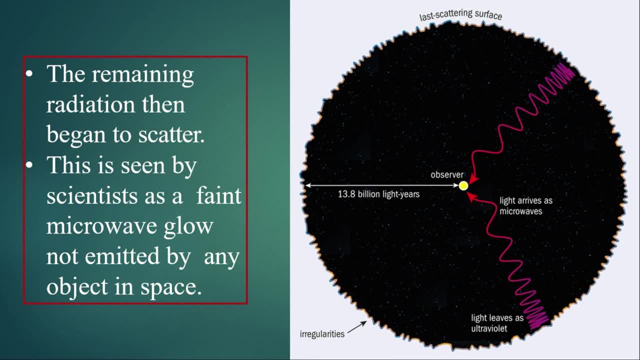 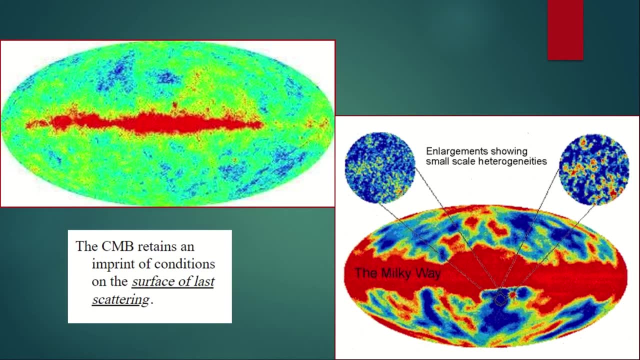 And up until now It is still observed- The cosmic microwave background Radiation. So the cosmic microwave background Retains an imprint Of conditions On the surface of last Scattering. So it became evident That it proved That there is a big bang theory. 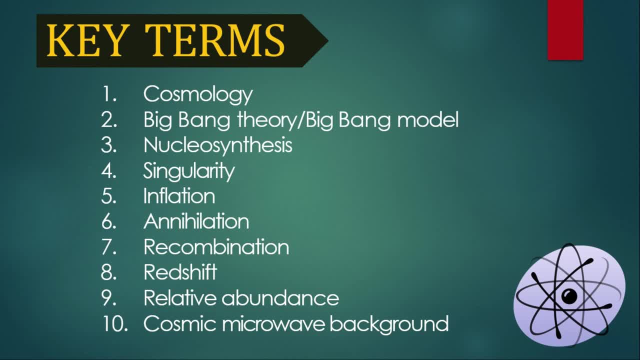 Let's have a recap. Today we have discussed About cosmology, The big bang theory Or the big bang model, How the universe evolved According to the big bang theory. We also looked Into the stages Of the big bang.